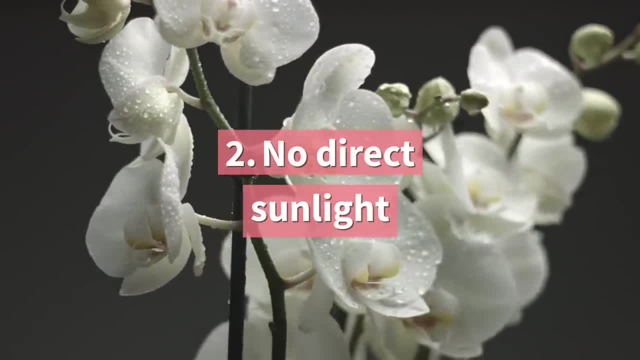 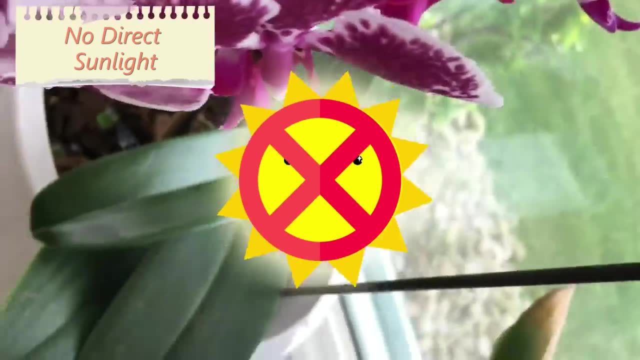 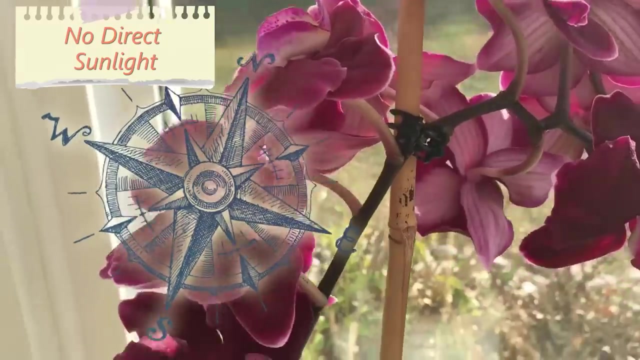 2. Know directly. Orchids are tropical plants, therefore, they do like light, but not direct sunlight. Therefore, it is recommended to place the orchid in front of a window that faces east or west. However, Phalaenopsis can face north as well. 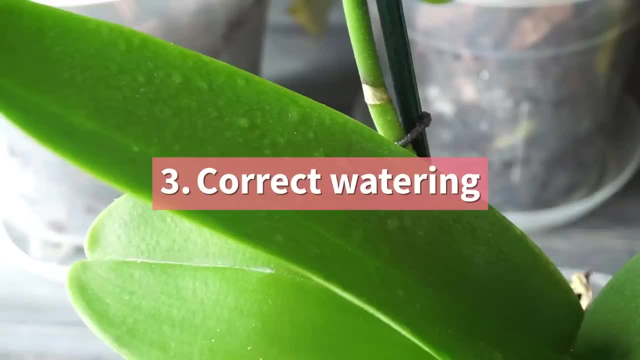 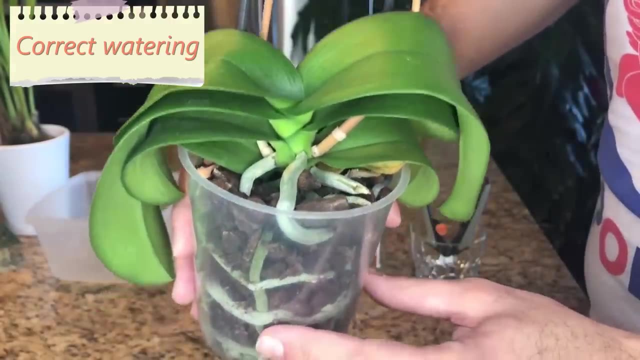 3. Correct watering. People make a common mistake by over-watering the orchids, Thinking it's a tropical plant and that it needs lots of water. In reality, there is no need to water your orchid more than once a week. 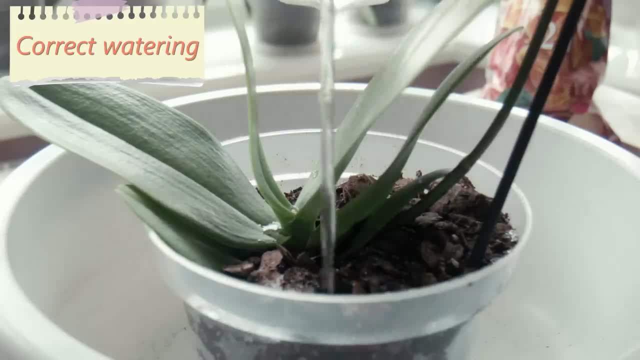 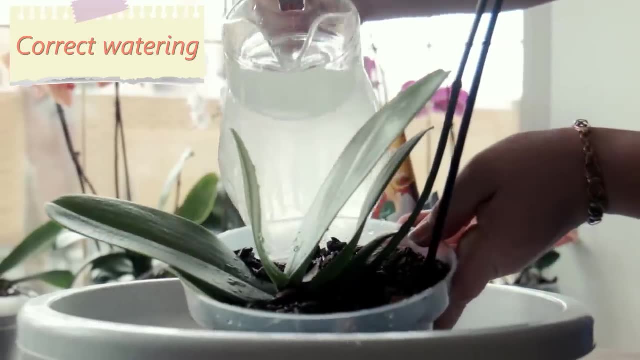 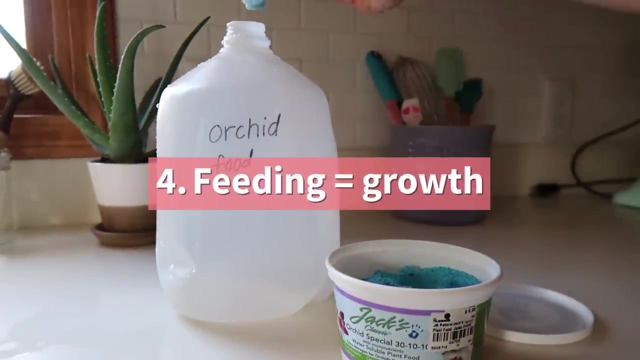 The best method to water the orchid is to submerge the roots into water for 20 to 30 minutes, or spray the orchid softly. Make sure the water is not too cold. 4. Feeding equals growth. Absolutely all orchids need fertilizers. 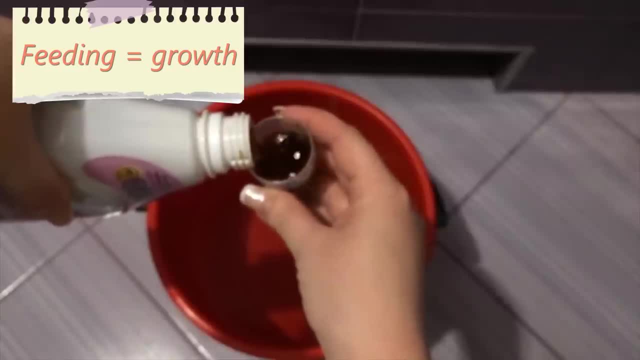 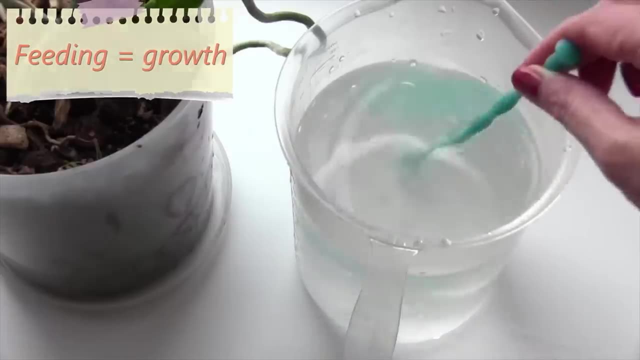 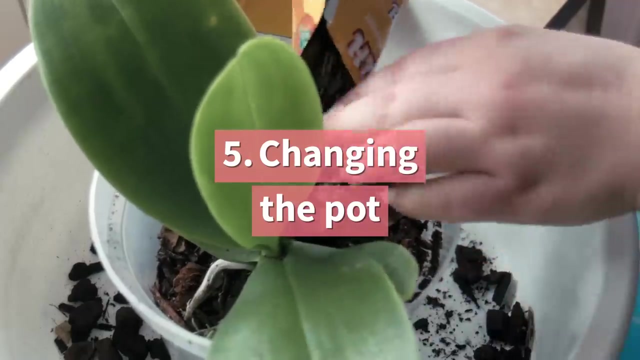 It is recommended to buy fertilizers that are specially designed for orchids. Fertilizers are added into water once a month during the active orchid growth only. 5. Changing the pot. Orchids need their pots changed every two years. 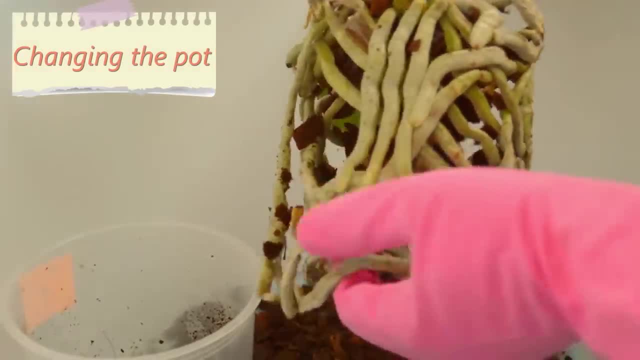 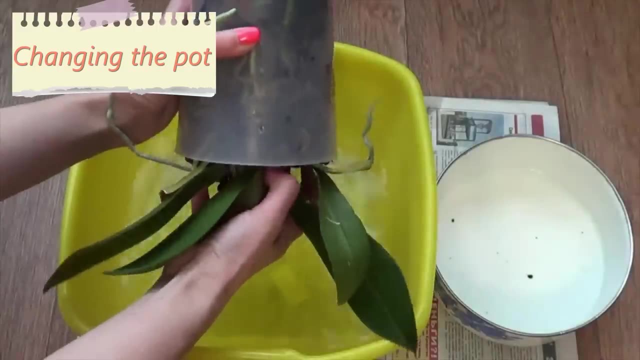 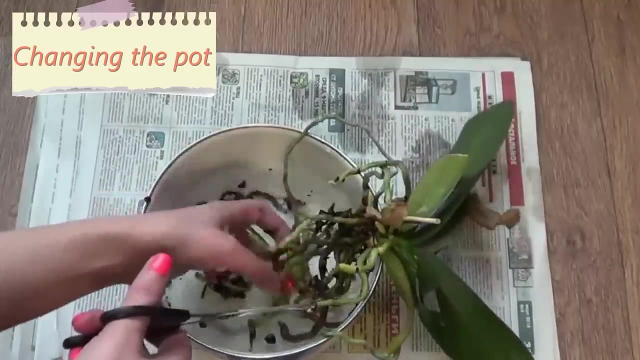 You have to be very careful because the roots could be damaged during the process. Fill the new orchid pot with new growing medium. Before moving the orchid, you need to trim all the dried and unhealthy parts from it. The end of trimmed parts must be sprinkled with cinnamon solution. 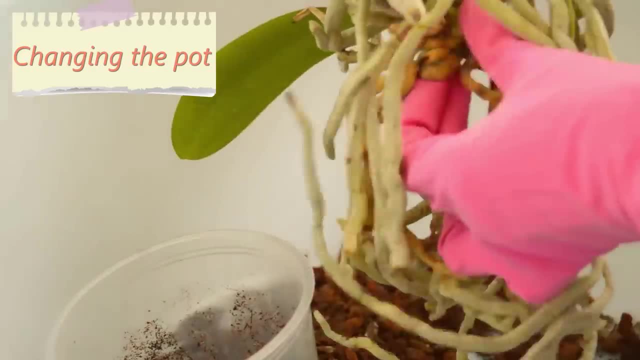 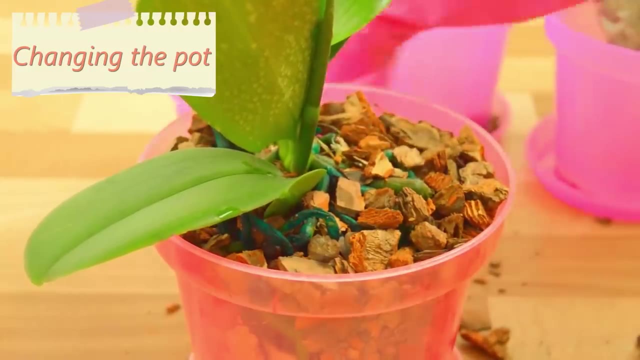 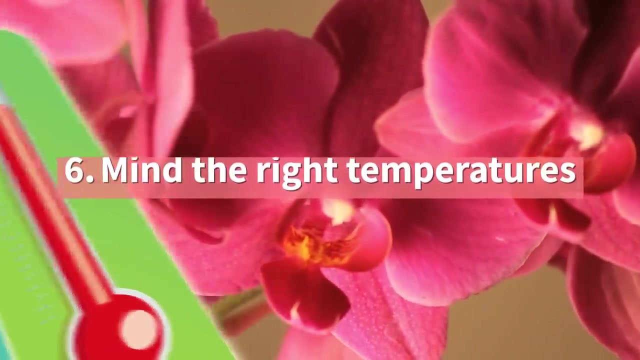 After repotting, water the orchid for three days straight and add the fertilizers in a month. 6. Molding- Molding is the most important step in the process. You need to be very careful: Do not overmold the orchid or it will be too hot. 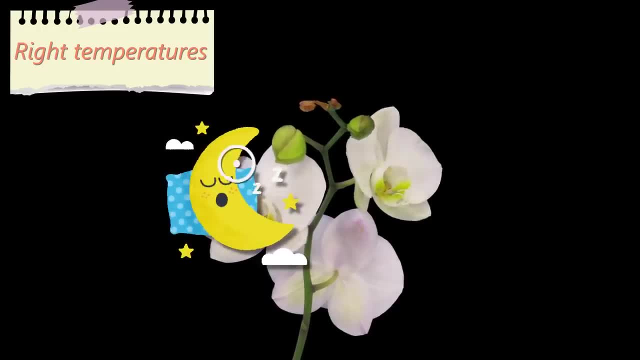 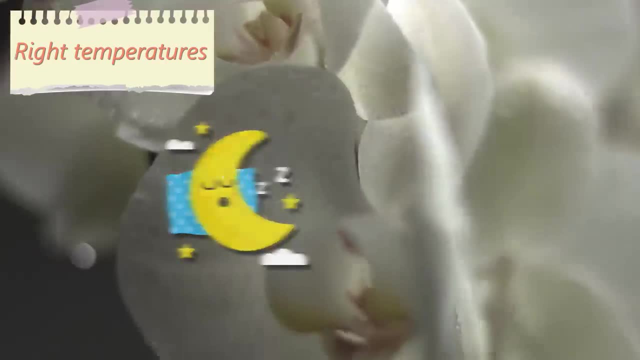 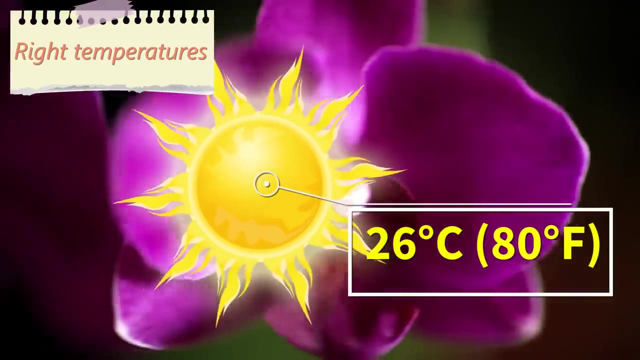 3. The right temperature, Mind the right temperatures. Orchids love mild fluctuation between day and night temperatures. At night, temperatures should vary between 12 to 18 degrees Celsius, 54 to 64 degrees Fahrenheit, and during the day the temperature should be 4 to 5 degrees Celsius higher.